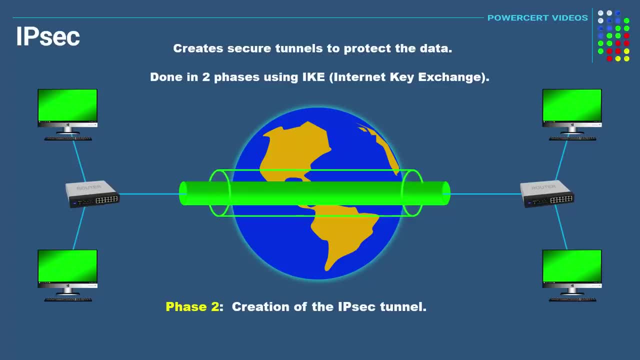 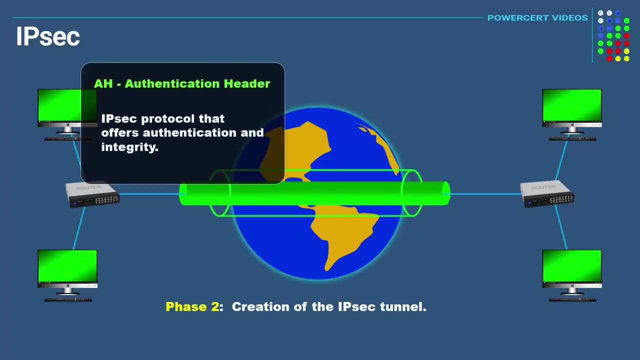 between the two sites. But before the data is sent, it needs to be protected, And this can be done by using a couple of different protocols. One is called AH, or authentication header. This protocol offers authentication and integrity, but it doesn't do any encryption. 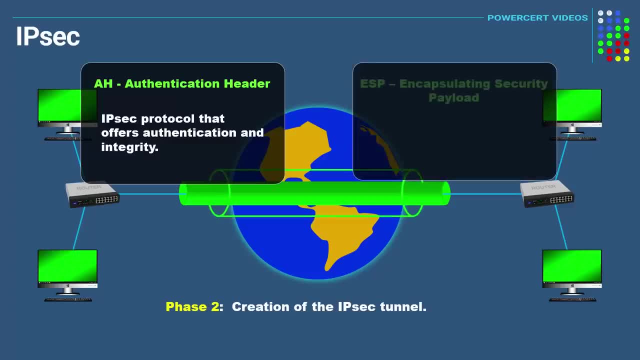 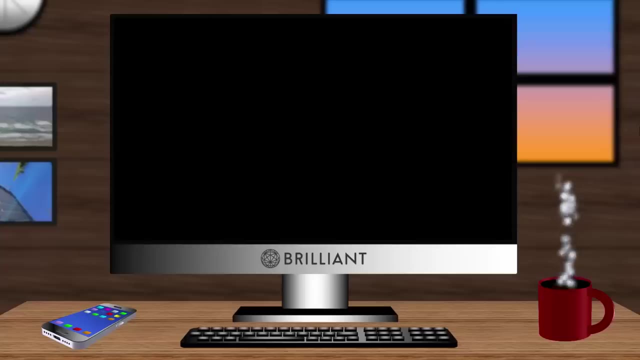 And because it doesn't offer any encryption. the other protocol, called ESP or Encapsulated, Isolating Security Payload, is the better of the two protocols. ESP does all three: It offers authentication, integrity and encryption. Hey guys, if you're watching my videos, you're obviously interested in learning. That's why I want to tell you about Brilliant. 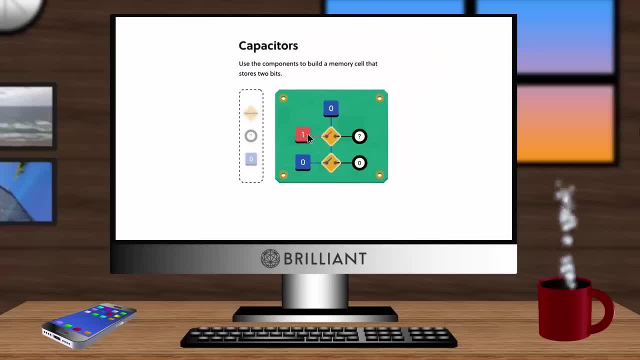 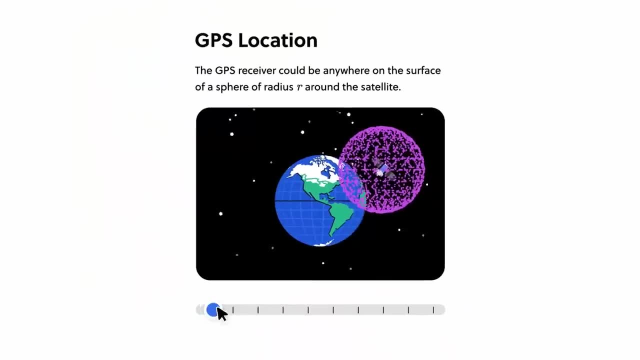 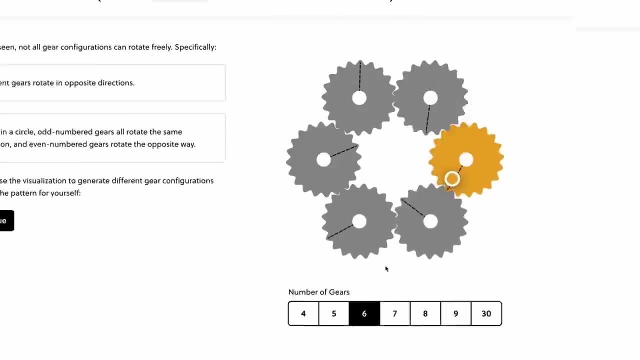 Brilliant is an online learning center where you can learn and master concepts in as little as 15 minutes per day, With thousands of lessons to choose from. their interactive lessons make concepts feel intuitive, so even complex ideas are easy to understand, And their real-time feedback and simple explanations. 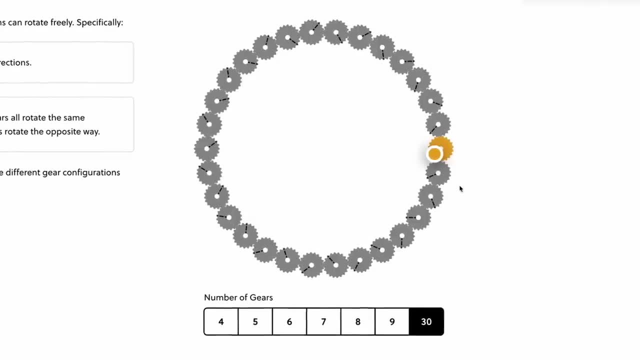 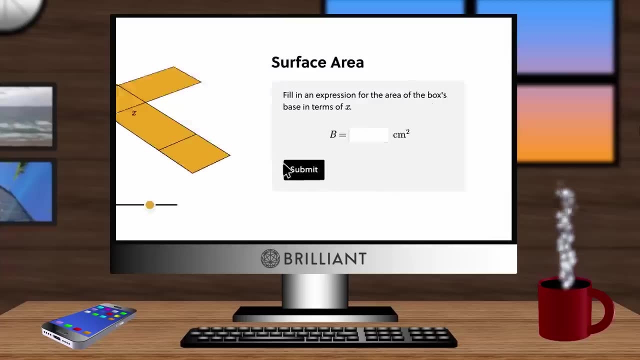 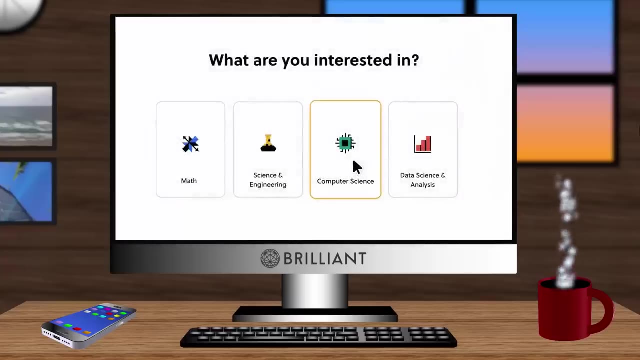 make learning efficient. Whether you're a complete beginner or ready to dive into machine learning and beyond, Brilliant makes it easy to level up fast with fun, bite-sized lessons, whether you're into engineering, computer science, data analysis or even math. Now me personally. 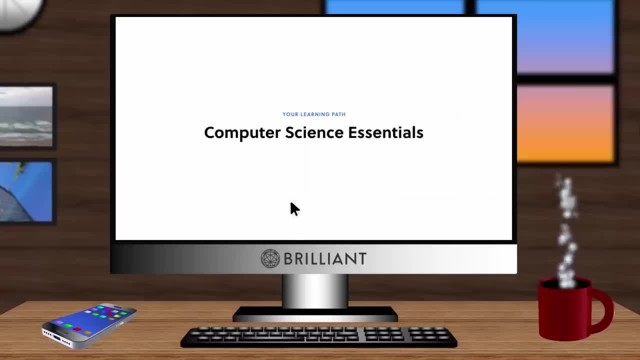 I'm taking the Computer Science and Programming course And, after completing my first four lessons, I'm going to give you a little bit of an overview of what it's like to be a computer scientist. The first two lessons: I was pleasantly surprised. The lessons are truly simple and, more importantly, 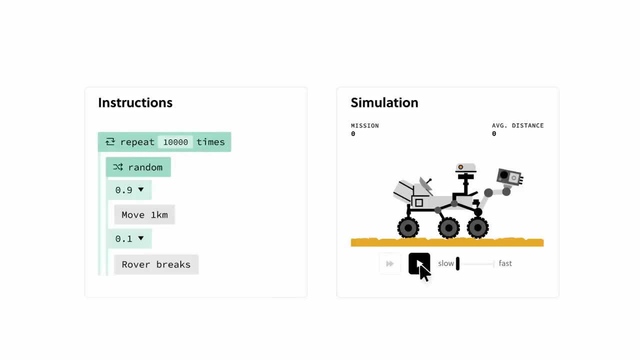 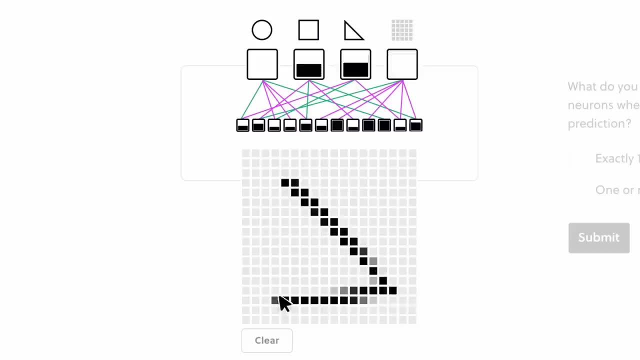 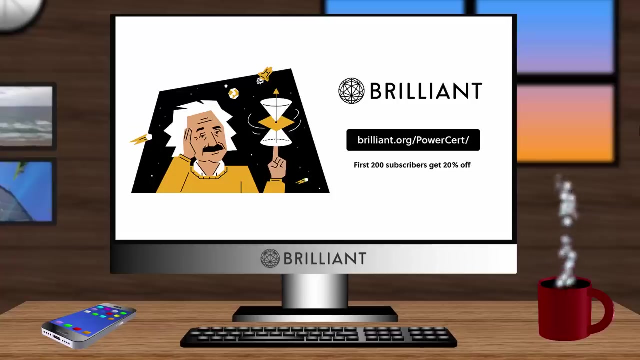 interactive, So you're not just reading or memorizing, but they teach you how to think and to problem solve. I actually find myself a little addictive going through these little lessons. So to try everything that Brilliant has to offer, free for a full 30 days, visit Brilliantorg. forward, slash PowerCert or click the link in the description. 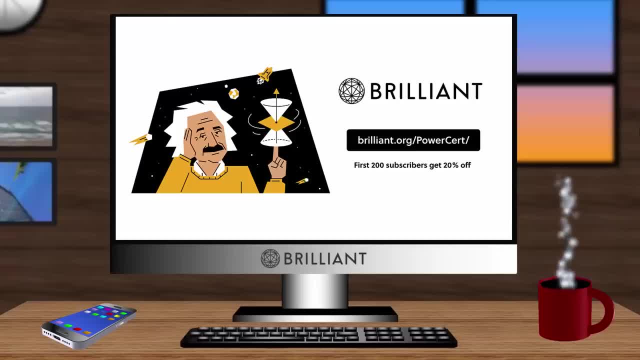 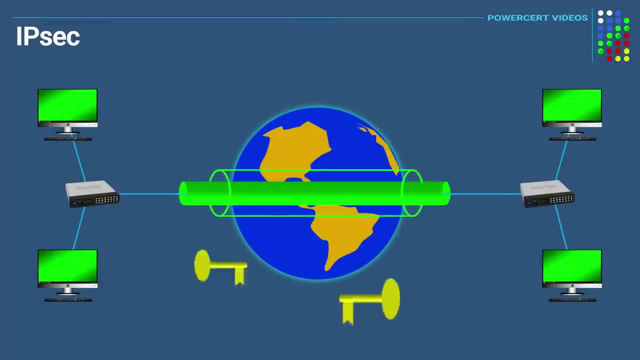 and the first 200 of you will get 20% off Brilliant's annual premium subscription. In order to use IPSec, both sender and receiver must share a public or private key. This key is what locks and unlocks the encrypted data as it travels across a network. This ensures 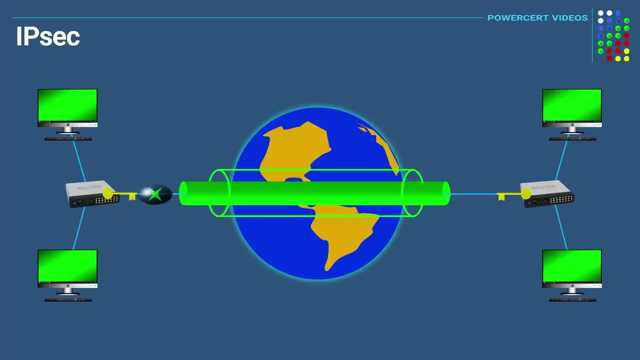 that the data cannot be read or tampered with. So when this site sends data to the other site, it'll use the key to encrypt, or, in simple terms, lock the data and then, as the data travels across the internet, the receiver.